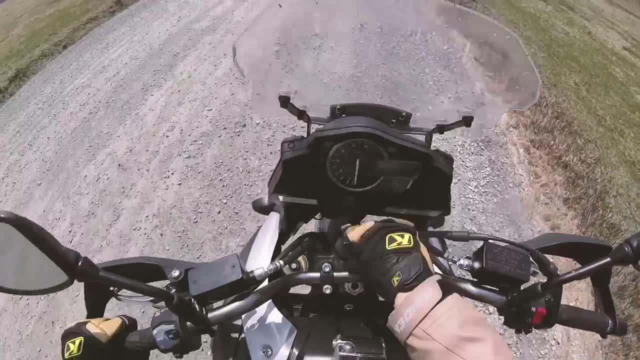 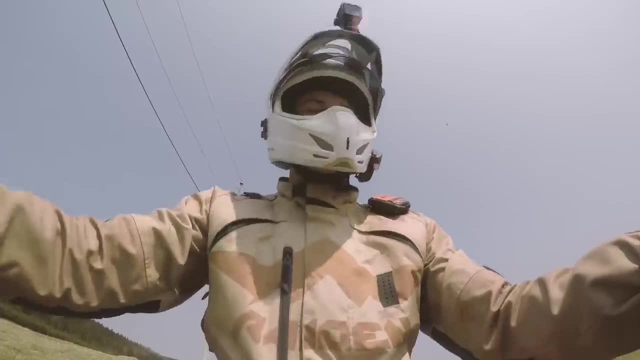 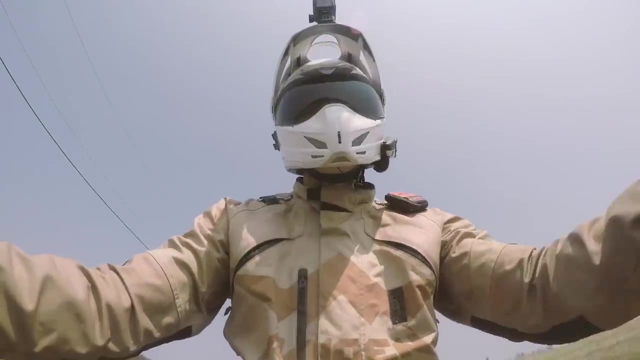 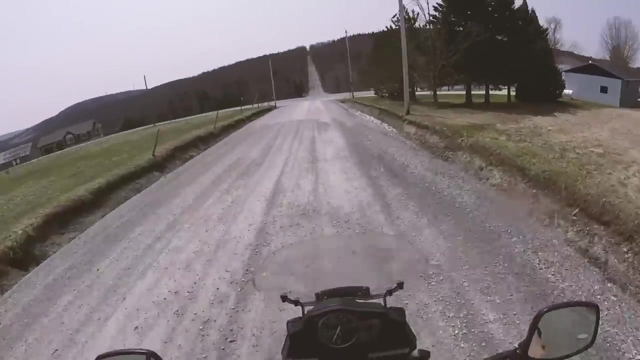 All right, let's get riding. All right, I love riding a windmill. We did a lot of this around the Gaspé Z and it's just like made me addicted man. It tends to just be so scenic and there's so many dirt roads. 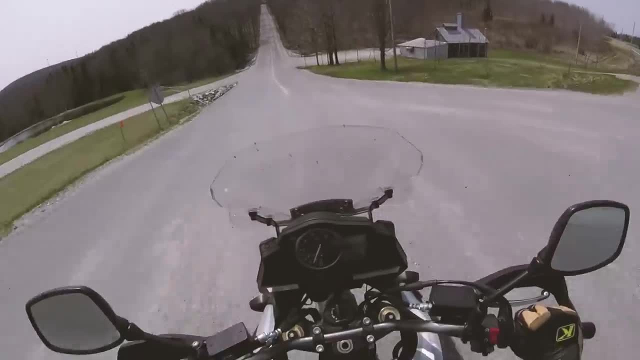 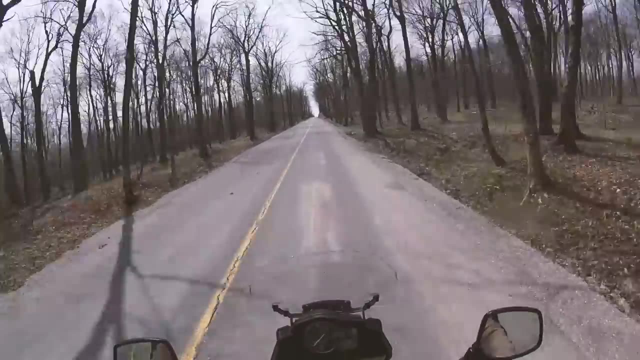 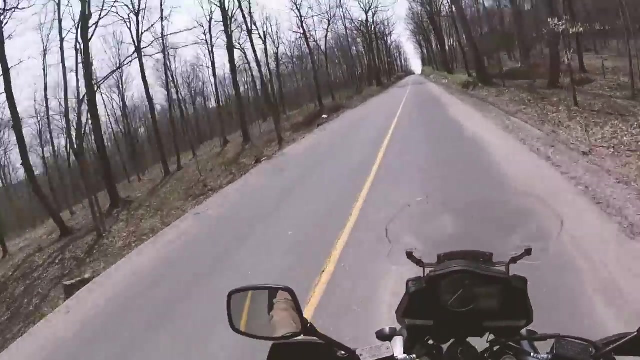 It's just awesome. Okay, I mean way to start. eh, I mean, look at this road, It's beautiful right off the bat, Okay. So I mean, as I was saying, people don't actually want to say how dangerous motorcycles are. 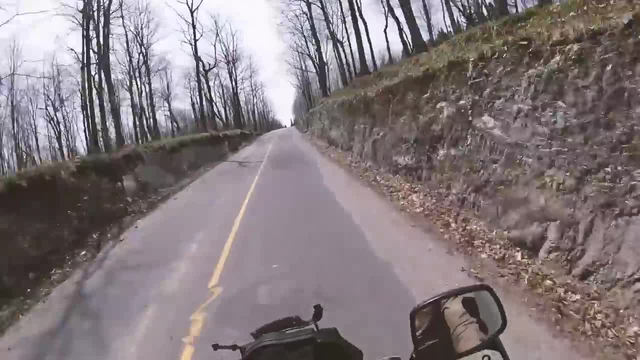 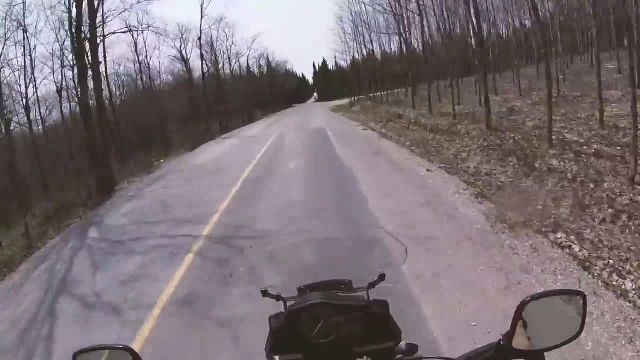 That's the topic of our vlog today. I went ahead and crunched the numbers. If you're watching this on the Fortnite website, you can find the math right below this video. If you're watching it on YouTube- too bad, too bad. I guess I'll link to it in the description. 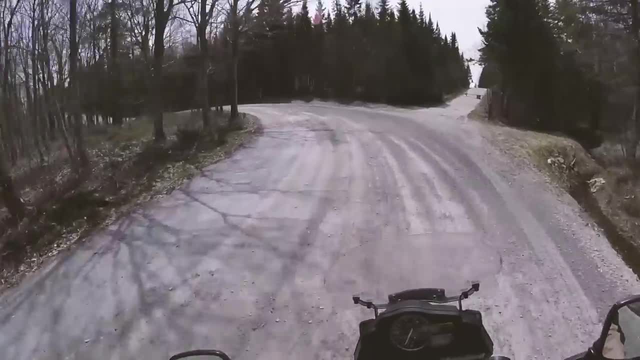 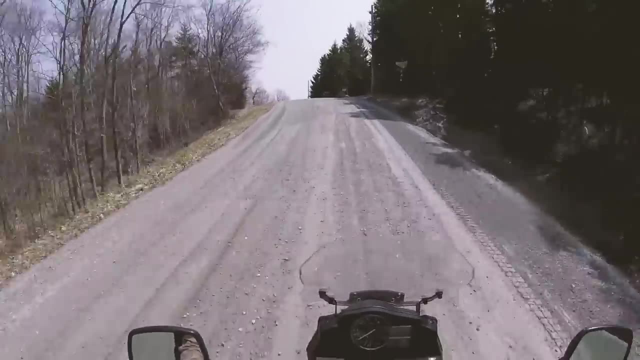 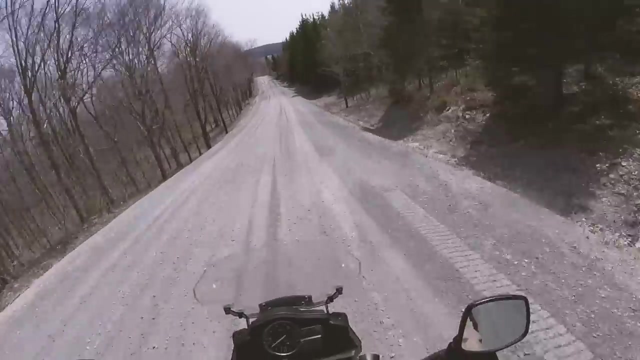 or something like that. But, oh yes, turned to dirt really fast. Oh, There goes the back end. So, yeah, I crunched the numbers. I basically looked at vehicles and then I did a experience. I didn't vehicle statistics in canada between- i think it was 2008 and 2013 and averaged across that time. 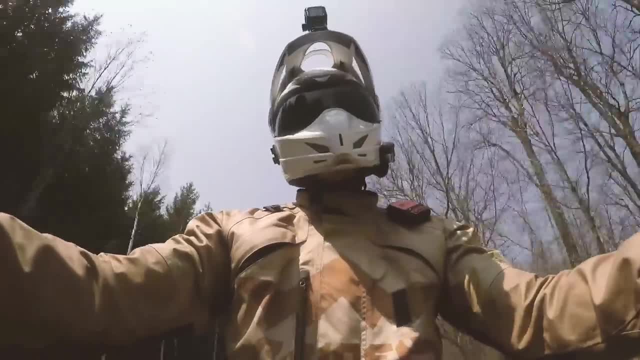 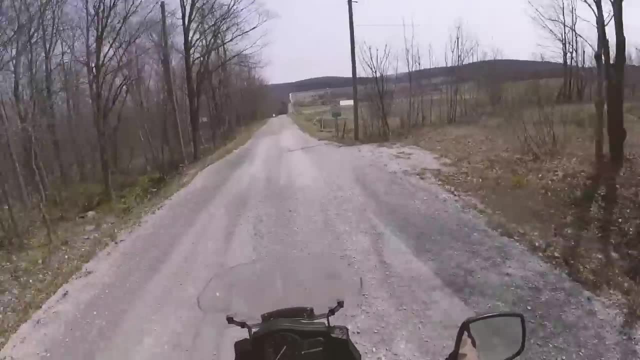 frame. i looked at light vehicle driver deaths- so ignoring the uh the passengers, and ignoring trucks and school buses and that kind of thing- and found out how many uh people died in car crashes on canadian roads. look at this, this is gorgeous, um. and then i did the same for 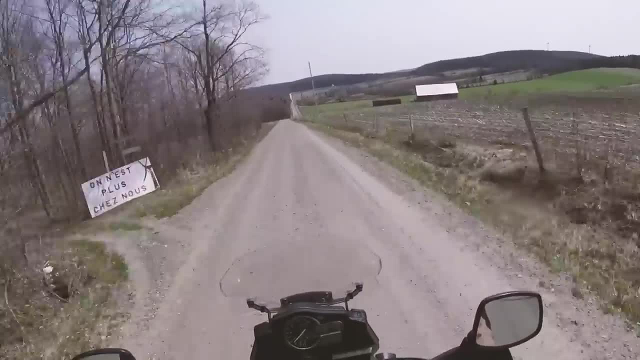 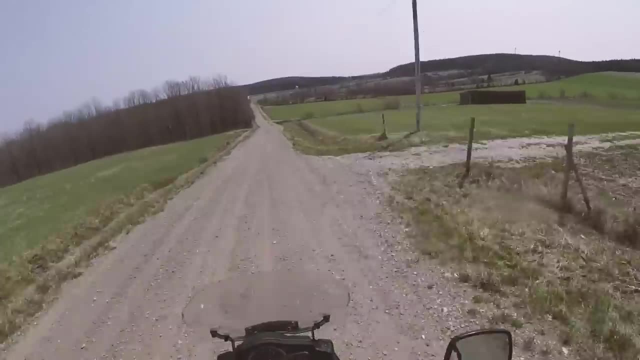 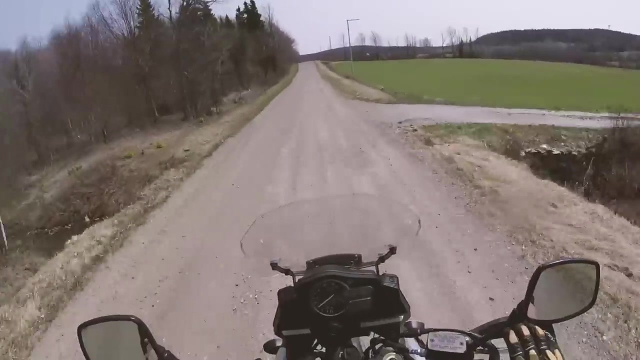 motorcyclists. i found out how many motorcyclists died on public roads in canada, again ignoring their passengers. i found out that the ratio was about 5.5 to 1.. um, oh, seems sad to talk about death and stuff on such a gorgeous sunny day in such gorgeous country. anyway, 5.5 to 1 for every. 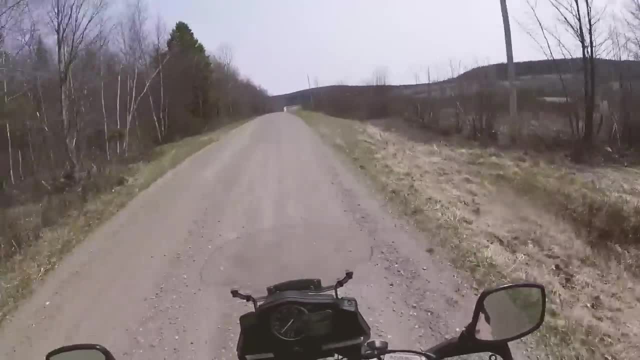 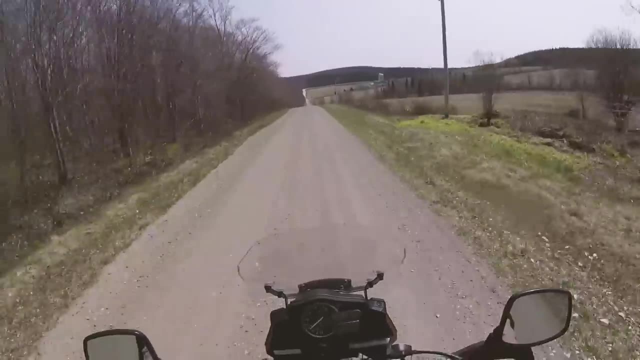 5.5 people that die driving a car or a truck or some kind of passenger vehicle on public roads. in canada, one motorcycle driver or rider dies um. so that was that ratio and then after that it was just a question of um looking at the number of registered vehicles. 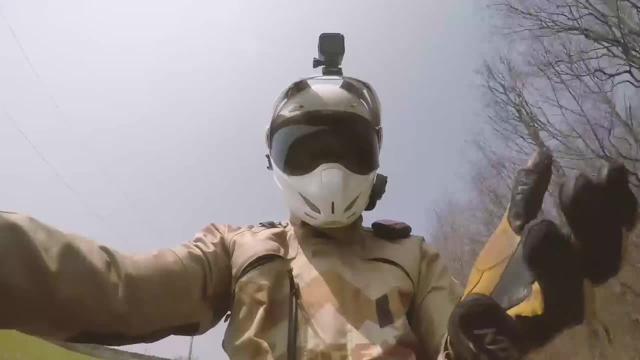 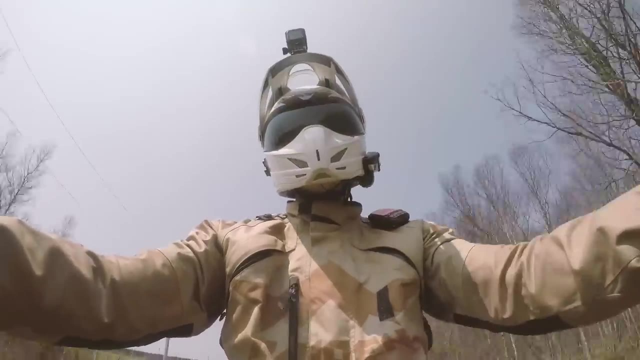 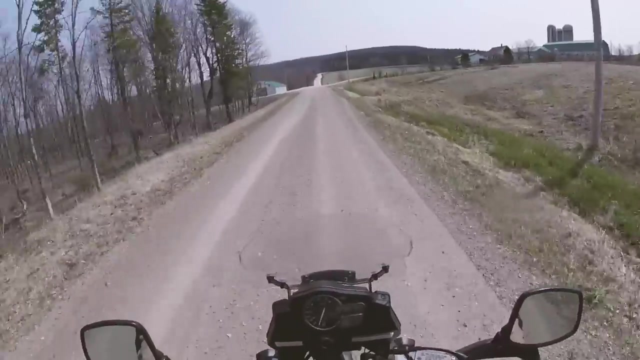 in canada over that time frame and the average kilometers traveled by uh a car and by motorcycles, then i could get the ratio 75 to 1, which is the ratio of light vehicle kilometers to motorcycle kilometers in canada. so for every 75 kilometers that the average canadian car travels uh a 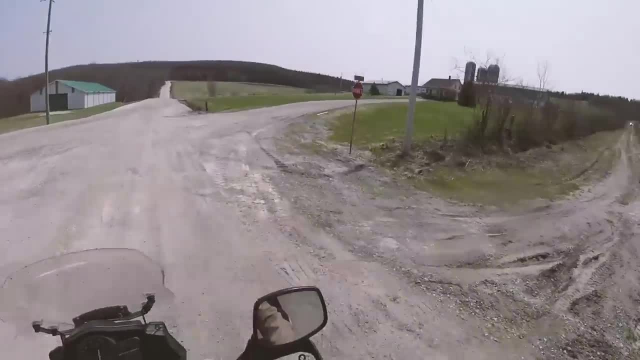 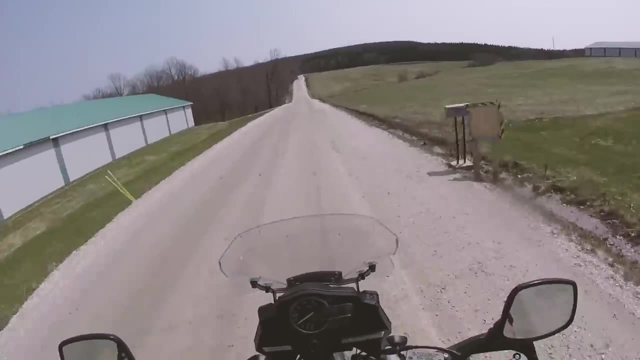 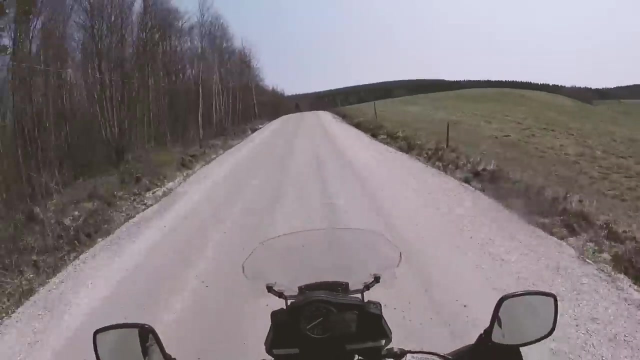 canadian motorcycle travels. one kilometer. is this stop sign for me? i don't know. oh, that it's so good, so i love dirt roads. you don't even have to break the speed limits necessarily, you just get like so out of shape, like fool around without any of the uh. 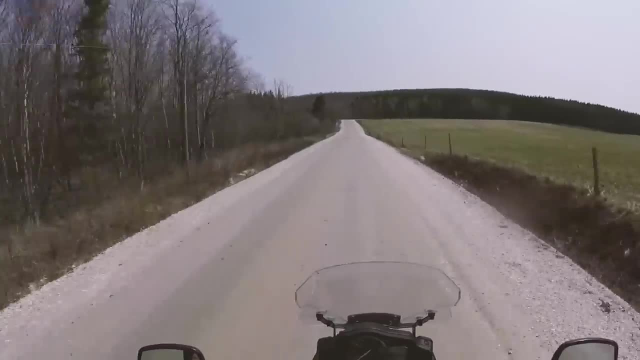 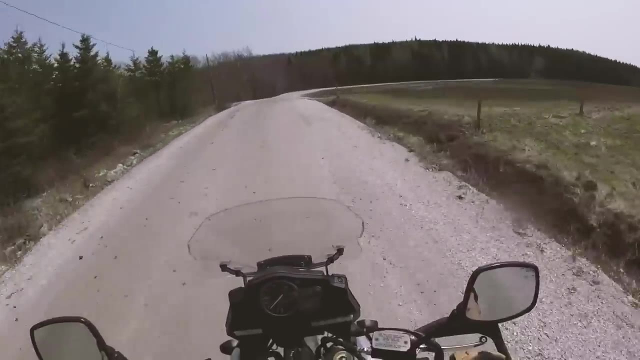 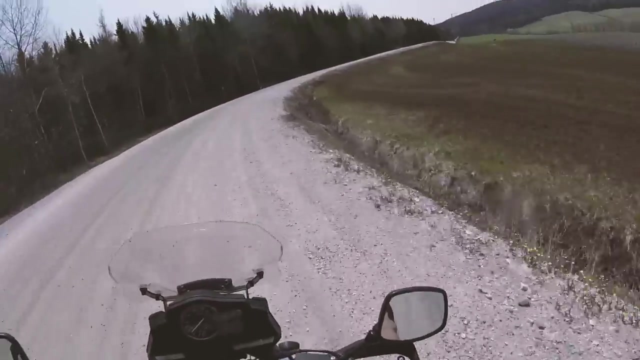 any of the real danger. so, yeah, danger, motorcycles. so 75 to 1 kilometer to kilometer and 5.5 to 1 death to death. you'd expect those ratios to be equal if driving a car and riding a motorcycle were equally dangerous, but they're not, so uh. so they're off by a ratio of 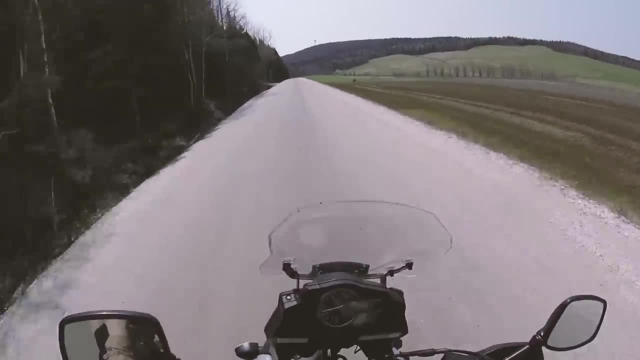 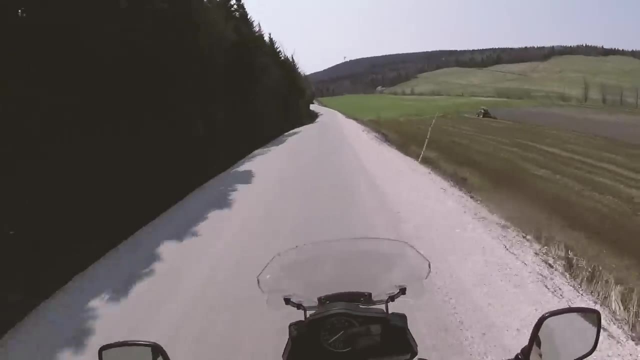 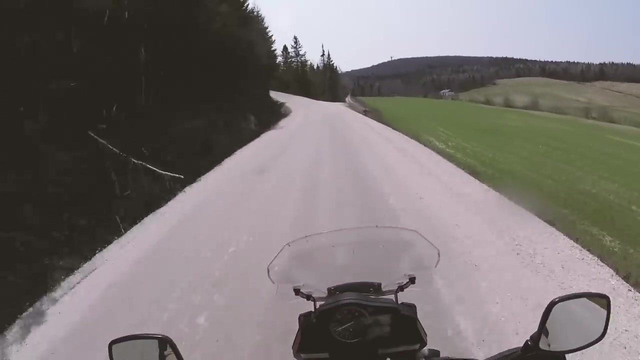 oh, hold on after this corner. oh, um, power drifts always distract me. um, they're off by a ratio of 13.5. uh, so basically that means that motorcycle riders are 13.5 times more likely to be killed in a car crash or vehicle incident. 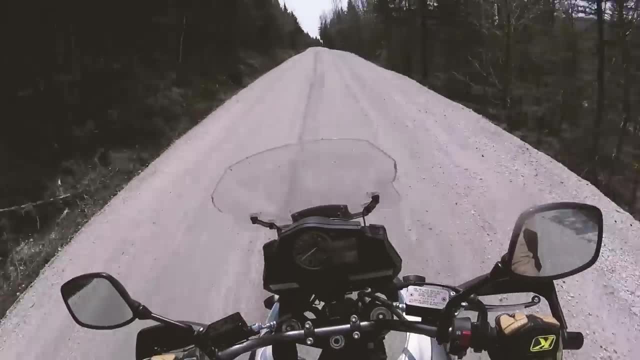 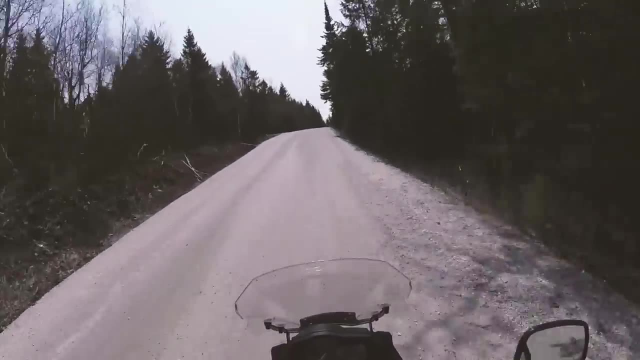 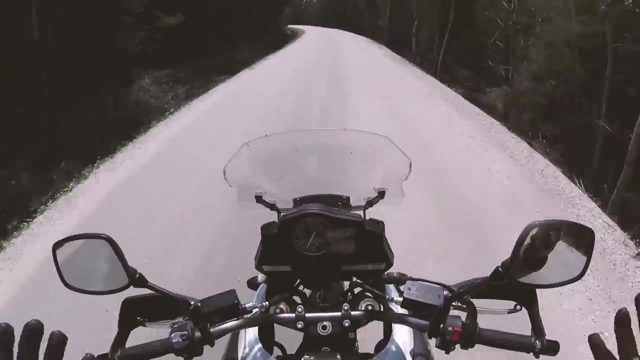 on public roads in canada, which kind of sucks, oh, but that cheers me up, um, Anyway. so the thing, though, is that I'm not dead yet. I've been riding around all day. I'm riding around out here, and I'm not dead yet. 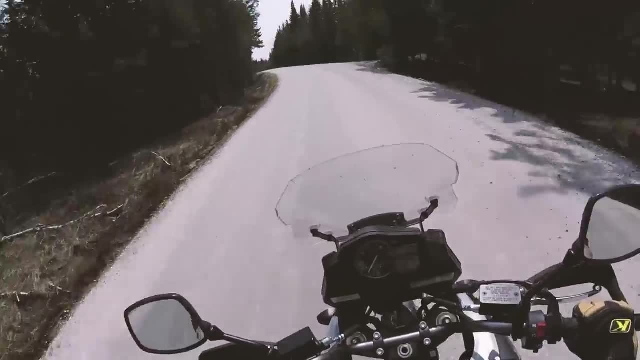 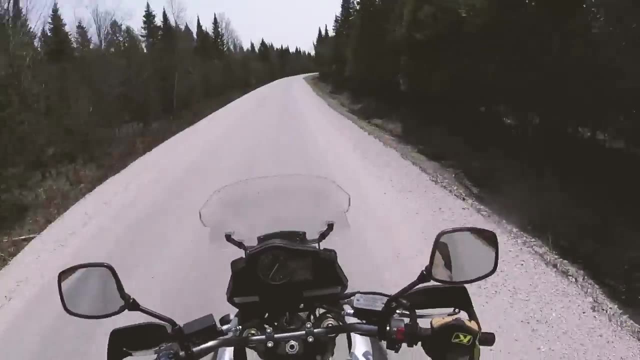 So maybe the number 13.5 isn't quite right. I certainly feel safer than that And, to be honest, it's true, I can actually feel safer than that and my number is probably much lower than the 13.5 average. 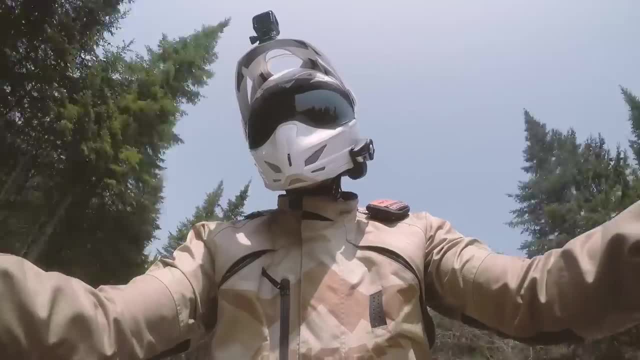 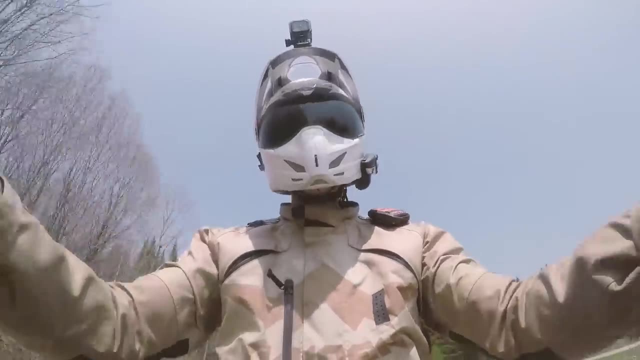 I'll tell you what I mean. So according to the Hurt Report, which is like that famous motorcycle study, it was about 50% of motorcycle accidents involve riders who have been on their bikes for less than five months. Well, I've been on this V-Strom here for about two years. 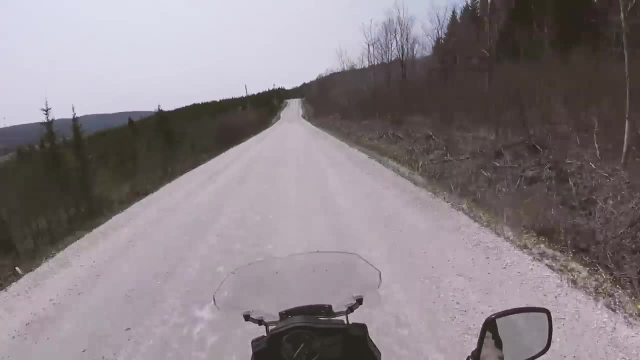 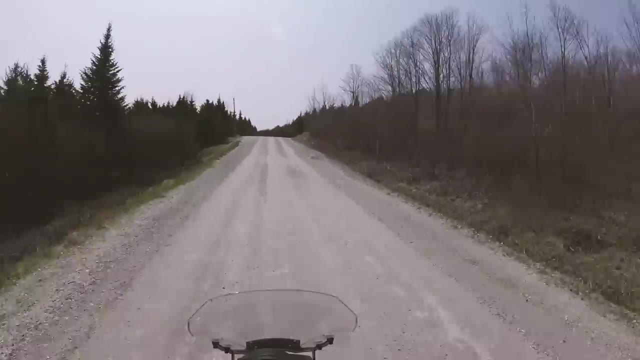 So I can officially drop my number 13.5 there. Oh, look at those windmills. Ah yeah, we're getting in nice and close to them now. This is good. I heard that the wings are about the size of a 747 plane wing. 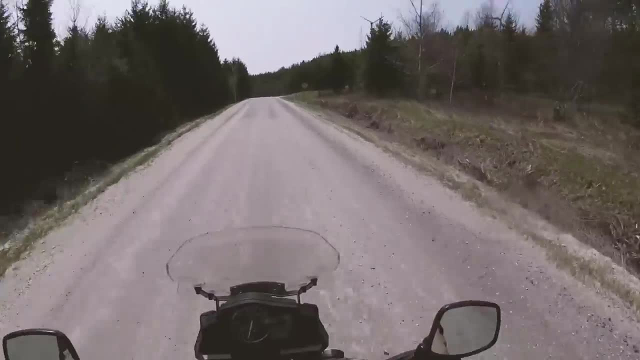 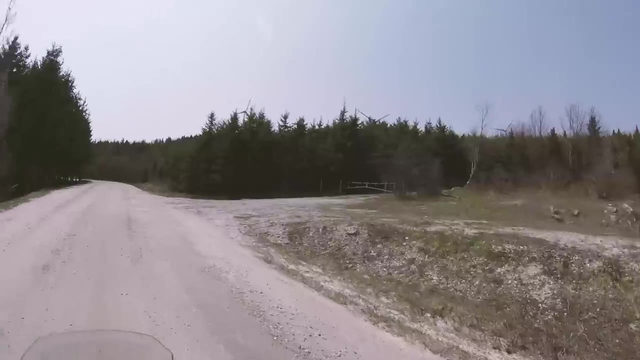 on some of the biggest windmills- I don't know if these are the biggest And the tips- We'll be going 200 miles an hour when they're fully, sort of rotating at the highest speed, which is really cool. Oh, look at that. 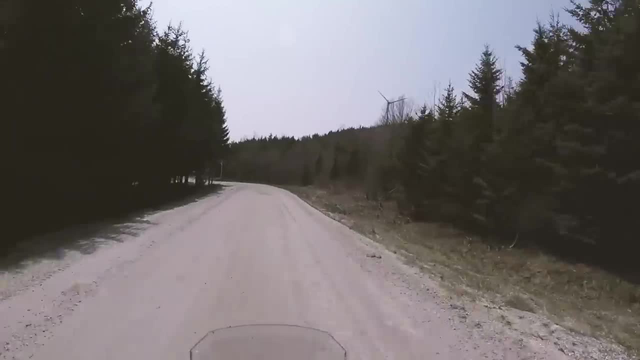 That is awesome. Oh, it looks like it's closed off though This one. yeah, it's closed too. That's a shame. See, in the Gatsby Z, you could like go right up to them. 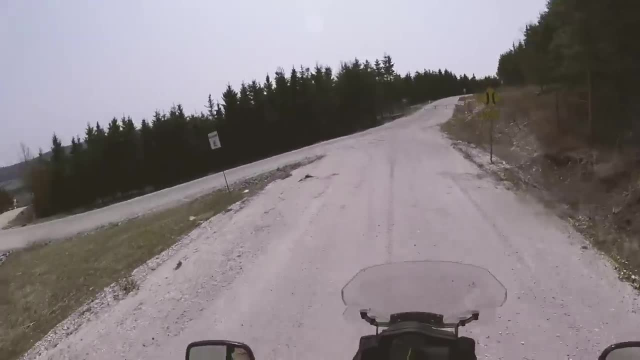 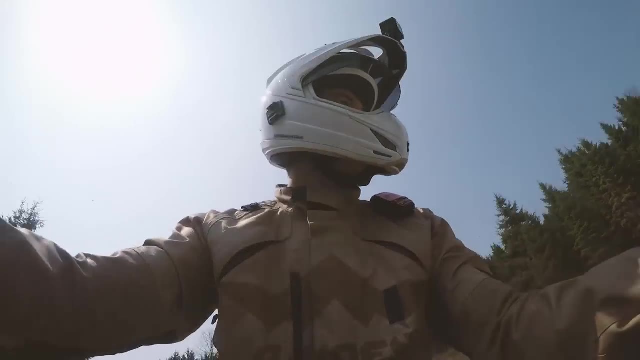 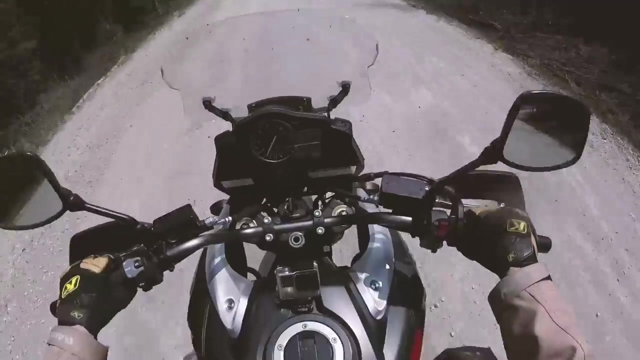 sit underneath them and stuff, But this is, um, yeah, private access, Bummer. Oh well, C'est la vie. I will probably ride Very happily anywhere they. let me ride up here, because this is absolutely gorgeous. I'm not going to complain. 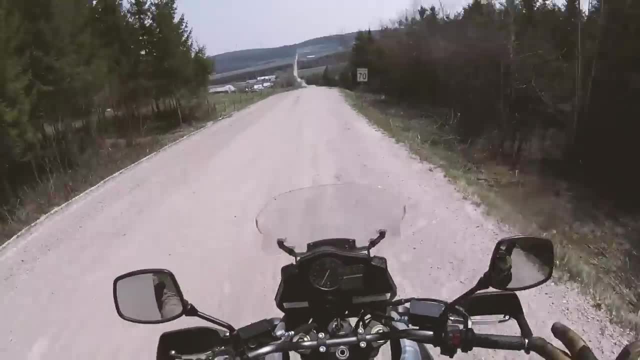 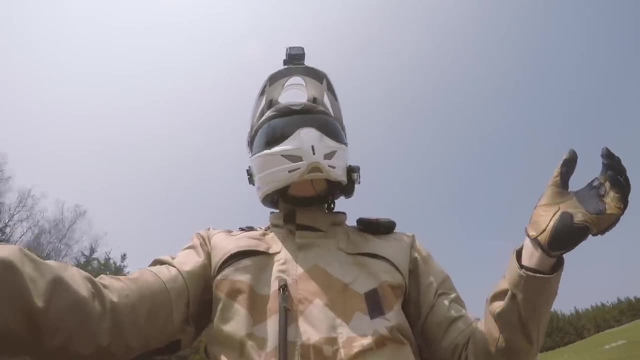 Oh yeah, amazing. So anyway, speaking of good news, we are dropping that number 13.5. by looking at how long you've been on your bike, You can also look at um. what was the study? In Ontario they did a study. 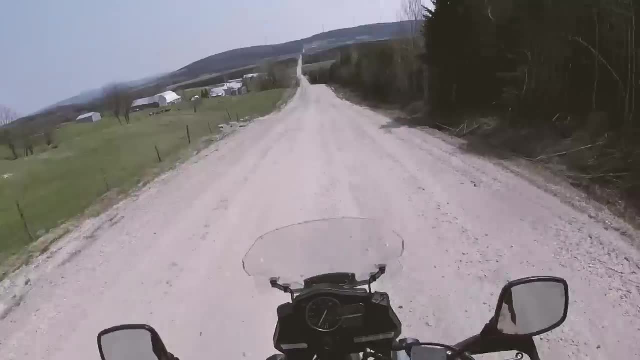 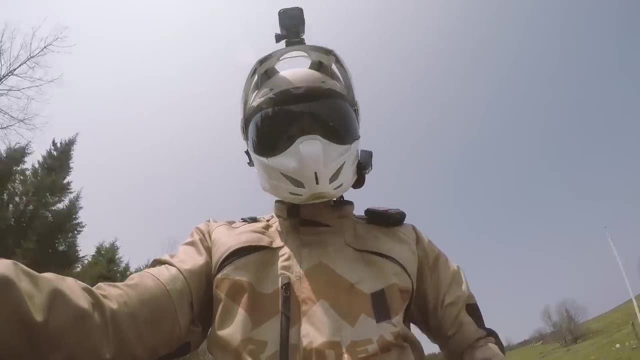 and it showed that about 25% of motorcycle deaths involved alcohol. So if you always ride sober- believe it or not, I'm riding sober right now, I always ride sober- Um then you can drop your risk factor there again. The same study of Ontario found that speed. 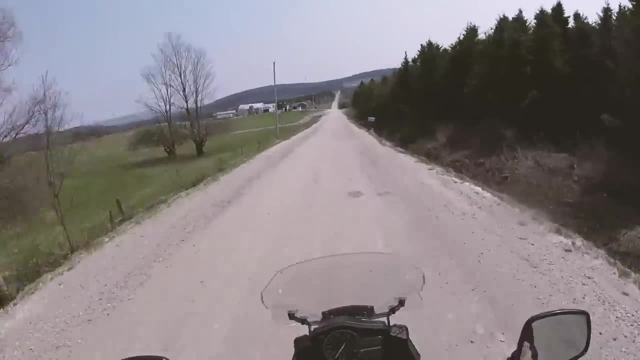 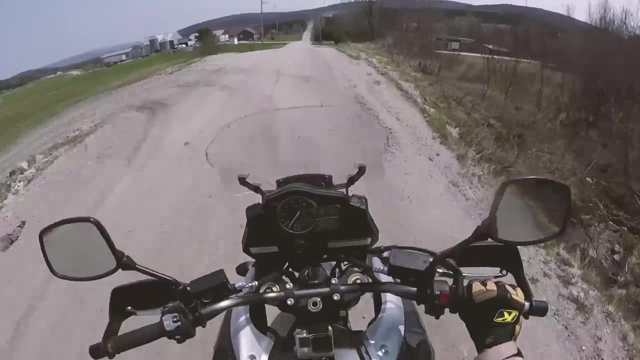 was a contributing factor in about 12% of motorcycle deaths, I think Um. so if you always keep it within limits, you can drop your factor there too. Um. in Quebec, uh, when they instituted mandatory motorcycle training um. 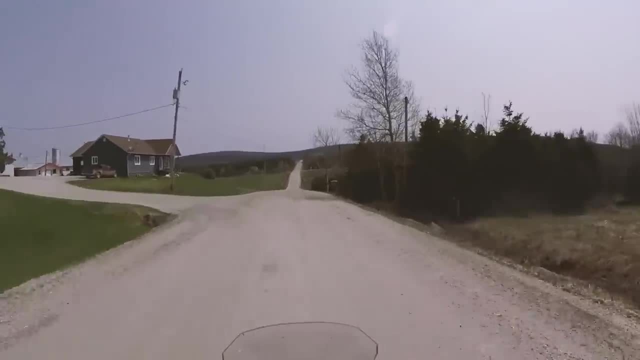 oh, look at this. Oh, there's just windmills everywhere up here: 1,, 2,, 3,, 4,, 5,, 6,, 7,, 8,, 9,, 10,, 11.. 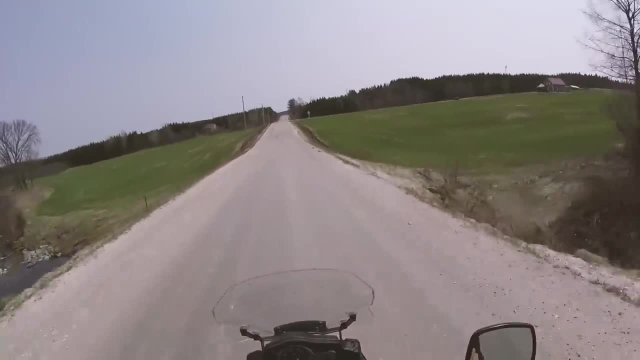 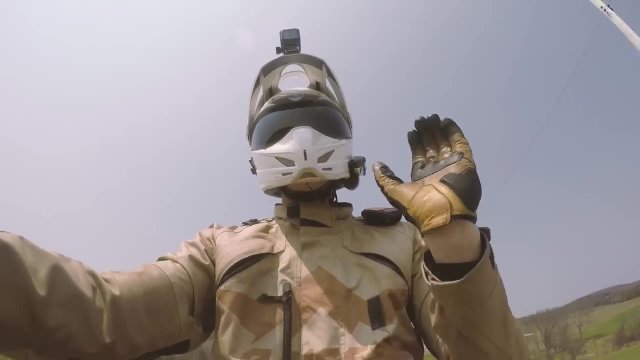 I wonder how big this array is. It's absolutely massive. Um so, when they instituted mandatory motorcycle training in Quebec, as I was saying, um 46% of motorcycle deaths like immediately fell off afterwards. So my recent graduation from motorcycle school. 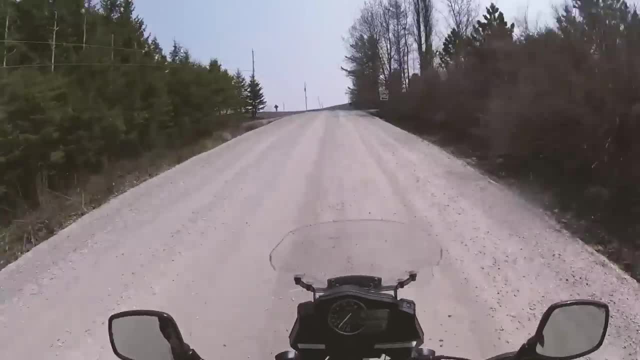 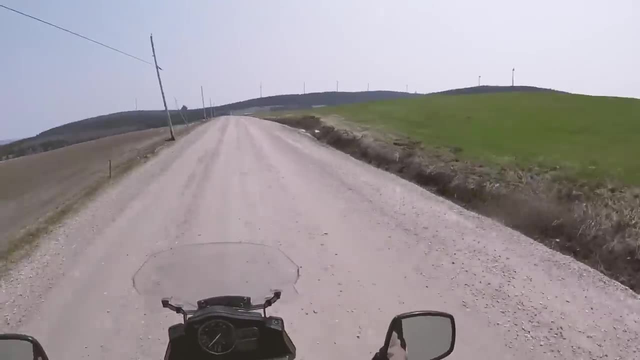 probably counts for something as well. Um, what else could we say? Uh, we could borrow from our friends to the south. In America they have stats on ABS systems. They don't have stats like that in Canada. Um, but uh, oh, it just keeps getting prettier. 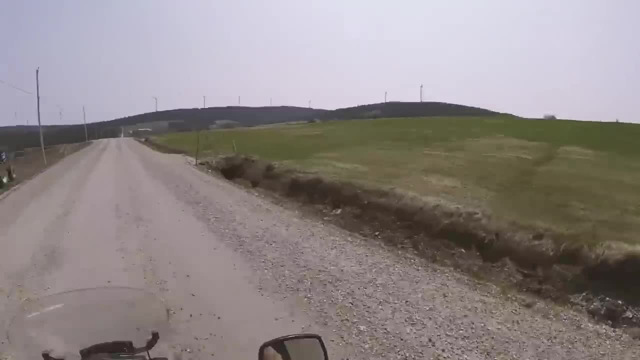 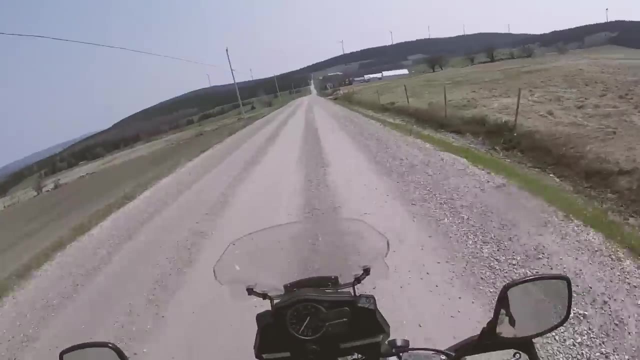 Ha, ha ha. Uh, I feel I feel so blessed to be riding around out here. It's unreal. Um, uh, what was I talking about? The states? Yes, if we're gonna borrow from the states, uh, they found there that I think it was 37%. 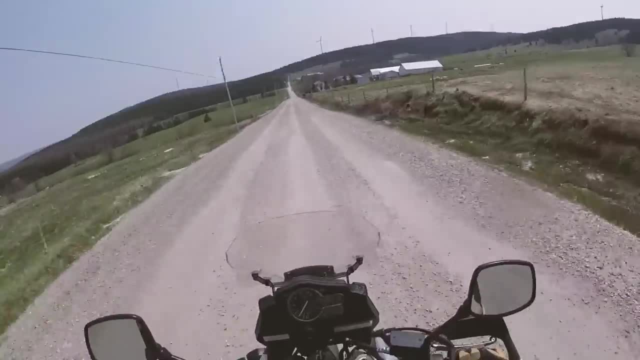 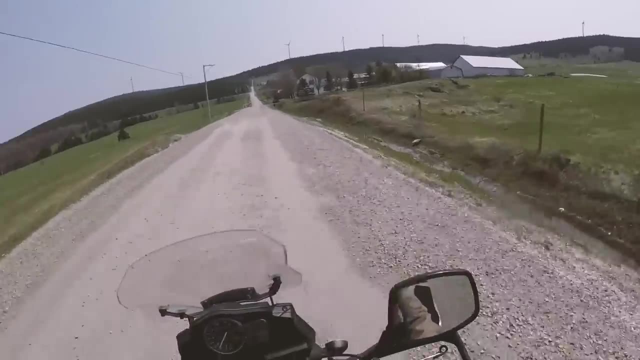 you're 37% less likely um to be killed in a motorcycle crash if you're riding a motorcycle that has ABS. Well, this motorcycle does have ABS. I found it kind of a cheeky way to turn it off when I want to sort of mess around off-road. 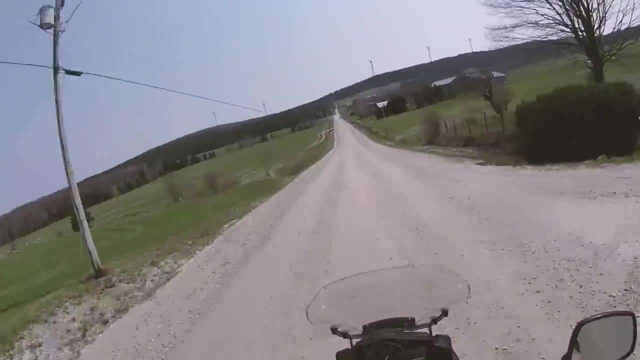 Um, but if I have the ABS on, that counts for something. Um, probably What counts for the most is ATGAT, All the gear all the time. I mean, it's kind of hard to put a number on it. 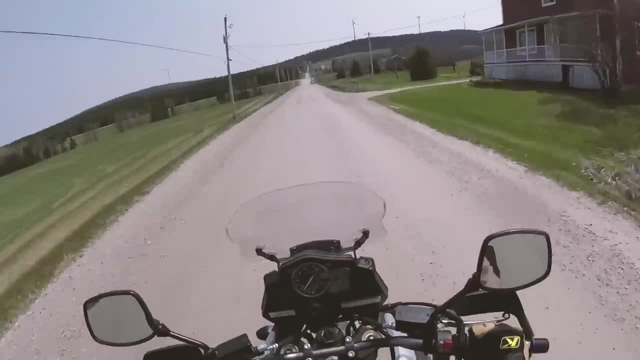 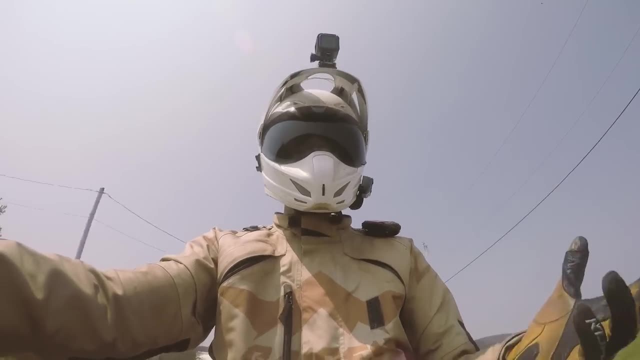 because everyone gears up differently. but not every Canadian has a full-face helmet, a fully-armored jacket, fully-armored pants, motorcycle boots, et cetera, et cetera. So if the average motorcyclist's 13.5 times more likely to die in a car crash, 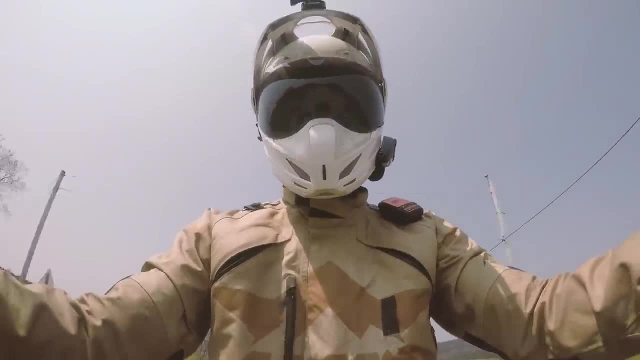 well, the average motorcyclist isn't geared up 100% all the time. So if I gear up 100% all the time, uh, well then that's gonna decrease my risk factor a bit more. I think that's probably. 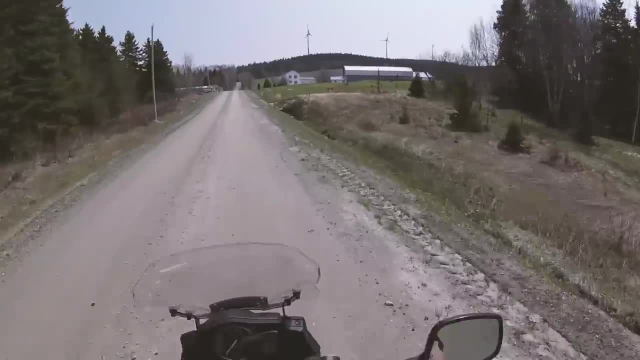 Well, if that's a cul-de-sac, um Uh, we'll see about that. I just want to keep getting close to these windmills. so if that's a cul-de-sac, uh, well, we'll see. 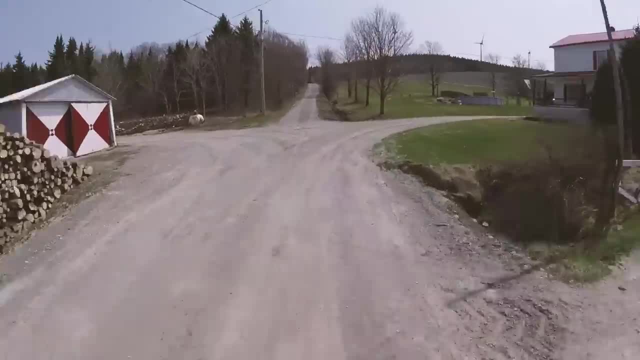 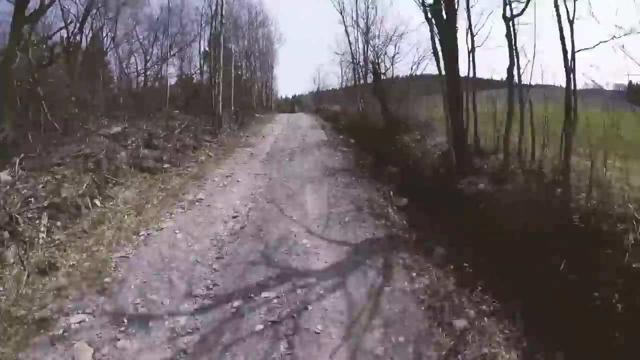 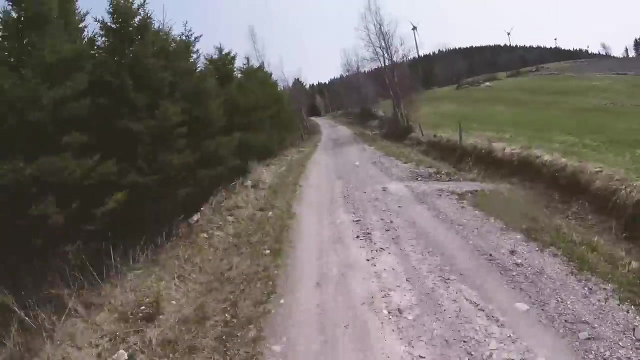 We will see, Woo, Can I come through here? I think so If I'm riding up your driveway right now. I sincerely apologize, Woo, But you have an absolutely stellar driveway. if this is yours, Woo, This is dope. Oh yeah, this is way more technical now. 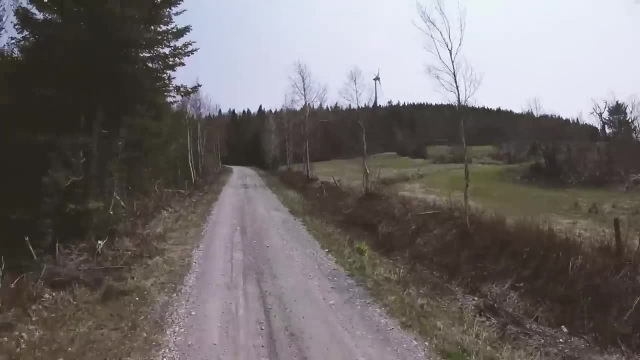 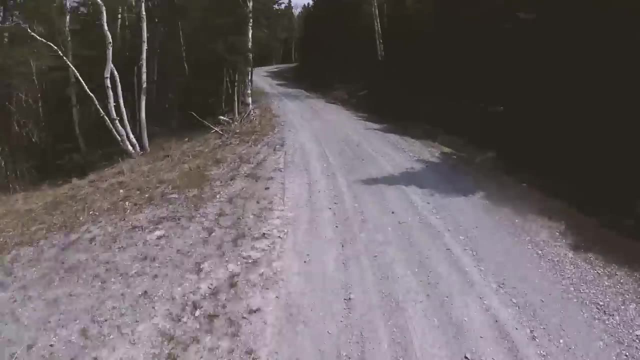 Look at how close we are to that. Oh cool, Apparently, you can park a minivan on top of the turbine there. Apparently, that's how big it is. It's hard to tell because it's so high up. Oh, this road's just getting better. 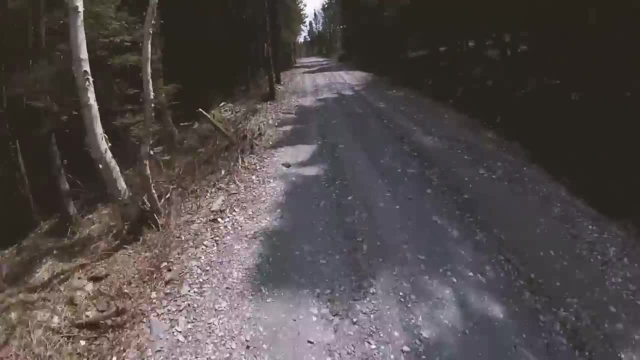 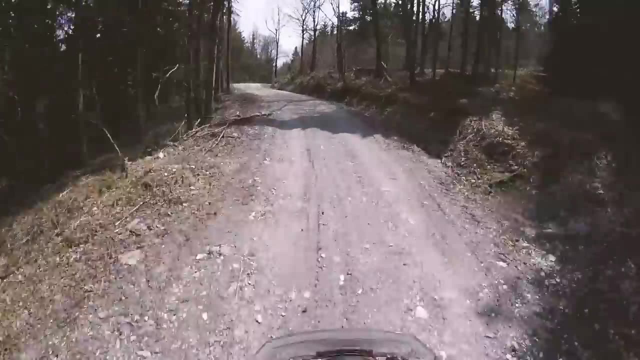 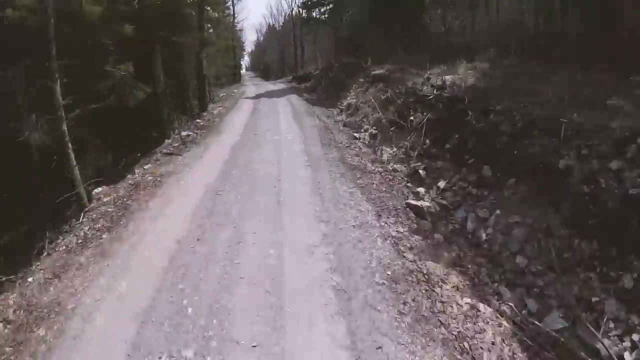 It's getting steep. Oh yeah, When in doubt, throttle it out. Yes Ugh, This is so good. So anyway, as I was saying, um you know, the number 13.5 kind of sucks. 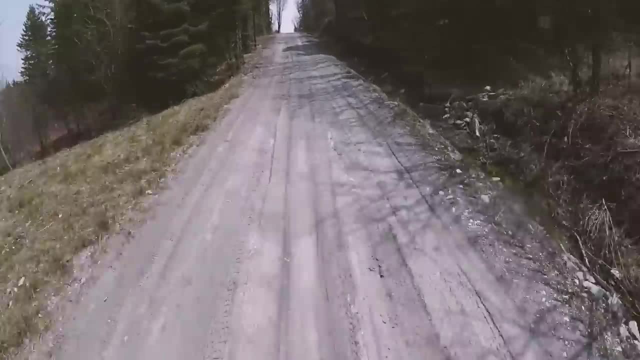 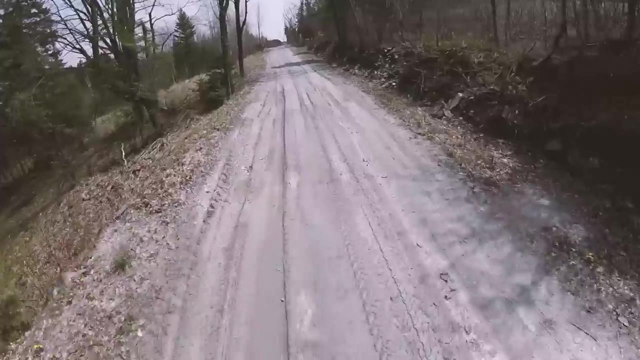 It sucks if we're that much more likely to be killed in an accident, but the good news is it's 13.5 for an average Canadian motorcyclist and you have a choice. You do not have to be. Ooh, it's getting slick in here.